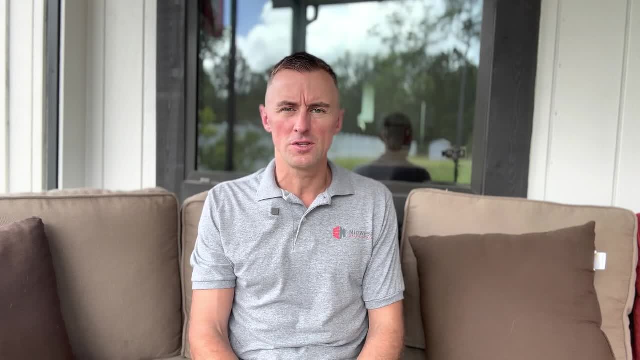 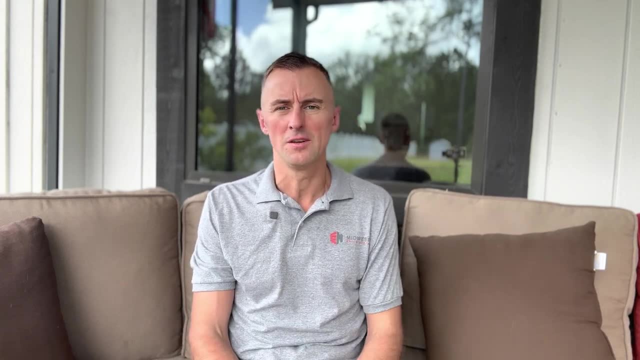 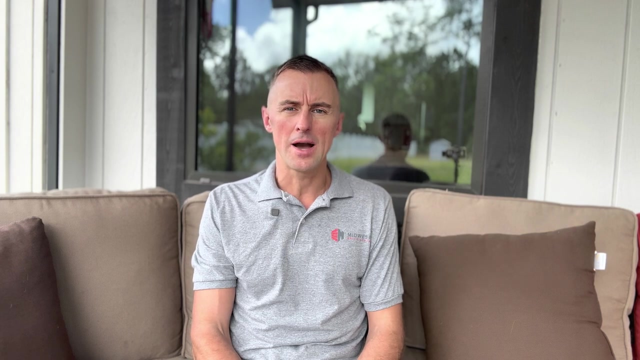 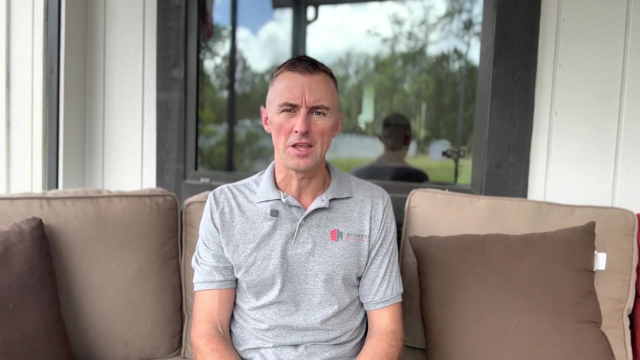 And what they're doing and other companies are starting to do is they're applying and marketing to. it's a stain, It's a brick stain, It's a concrete stain. So I wanted to identify the difference. First and foremost, inorganic mineral pigments are not compatible with ingredients such as propylene, glycol and other fillers that they use to achieve these colors. 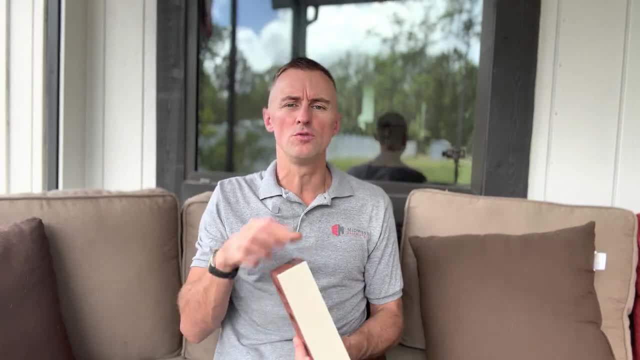 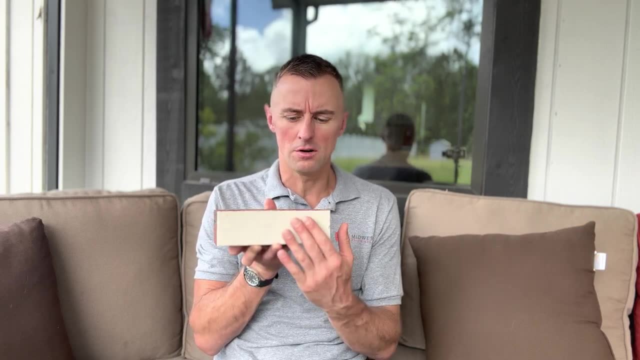 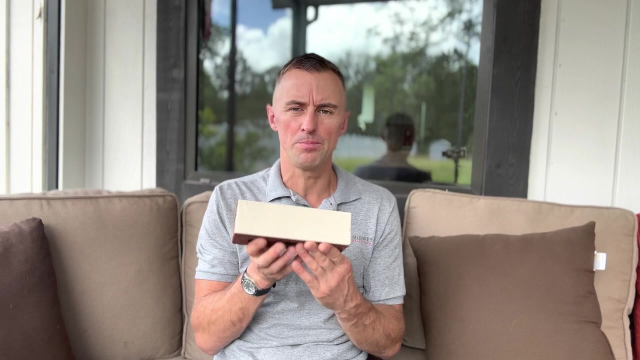 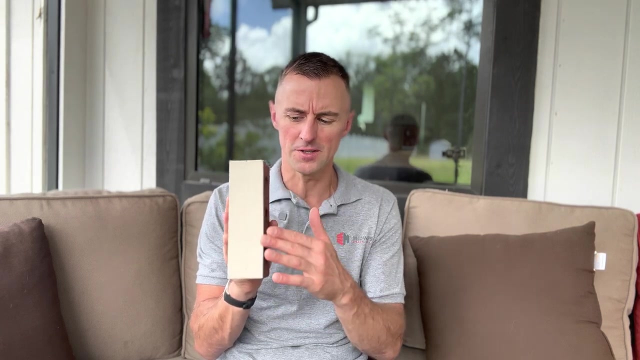 So when we talk about the products that we use- so, for instance, here's a beige tint- You're going to achieve more of a matte color versus a shiny like a sheen, versus using a traditional paint, for example. So what you're wanting the product to do is soak into the actual surface, not put a bond over it, And that's where the marketing goes a little bit backwards. 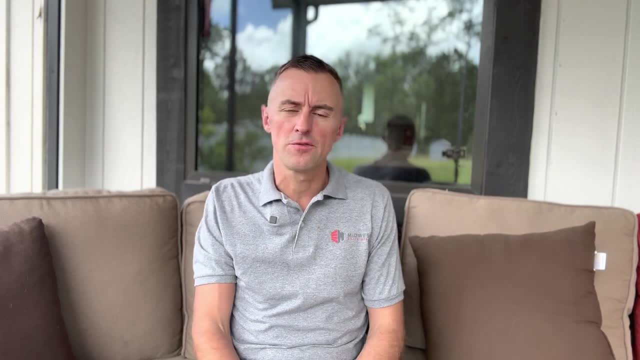 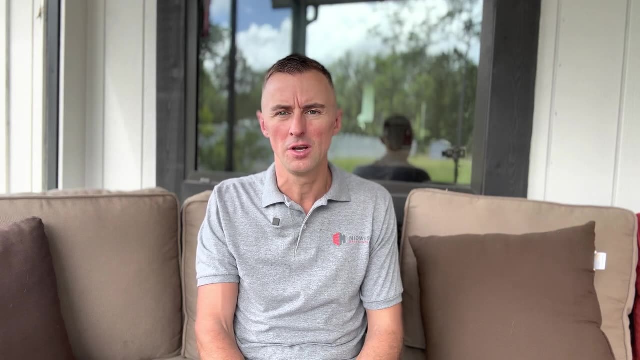 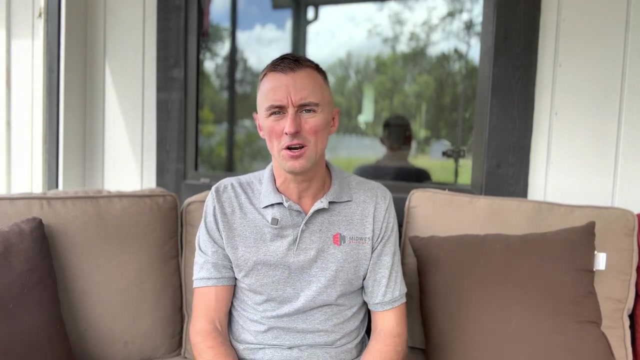 And I always ask folks to ask for a water vapor or permeability tests just to see how the paint reacts in the laboratory, And we can market this 50 different ways. There's really no oversight. There's no one that checks these companies. 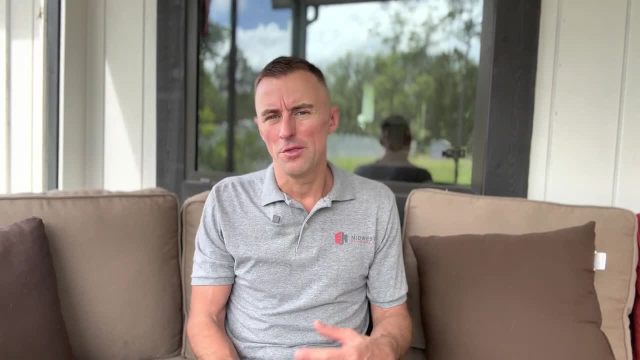 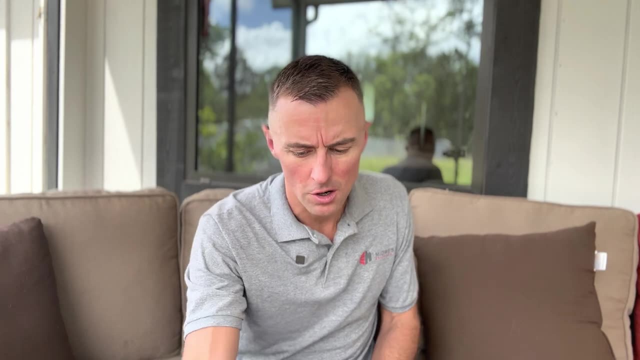 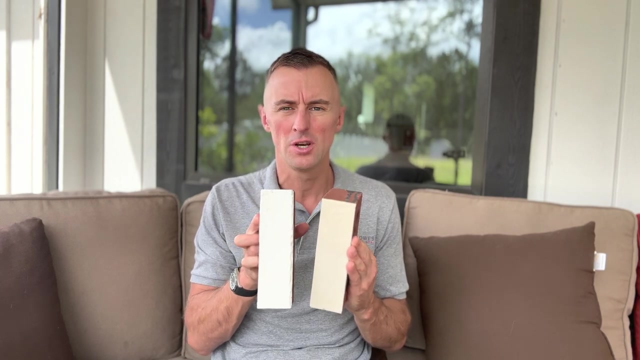 And when you start marketing inefficiently, that's when people get confused and they're like: what about this product? What about that product? So, just to keep it simple, All right. So our stains. I'm going to show you a few colors here. You got a beige and an alabaster. for instance, a pH in a potassium silicate stain which, just, it's a water glass with inorganic pigments. 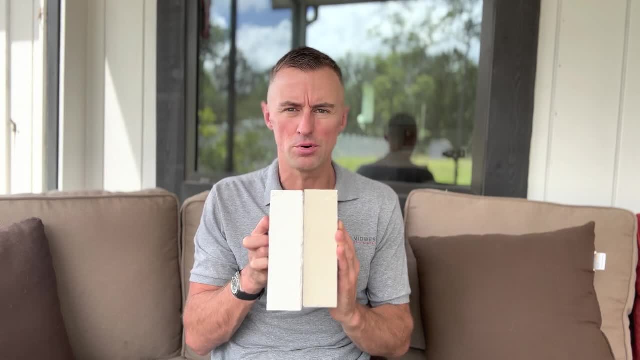 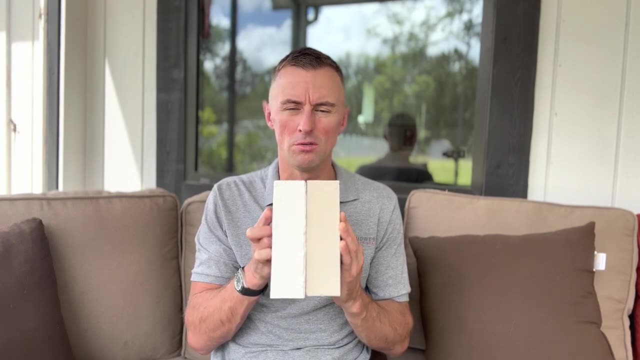 Let's just keep it simple. When you use our product, or we use our product on our services, a pH of 11 to 12 is achieved. It's alkaline, which means no mildew or algae are going to grow on top of this surface. 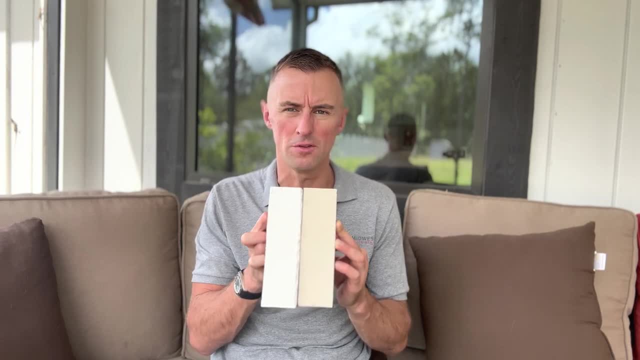 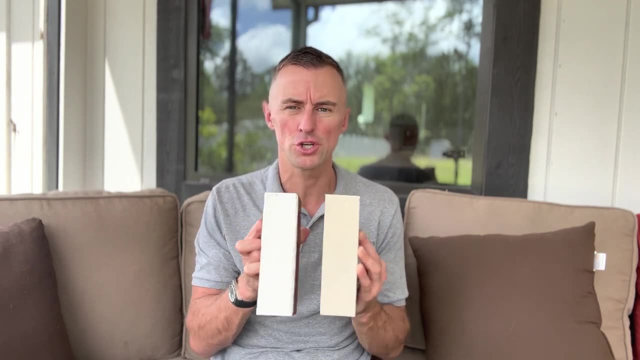 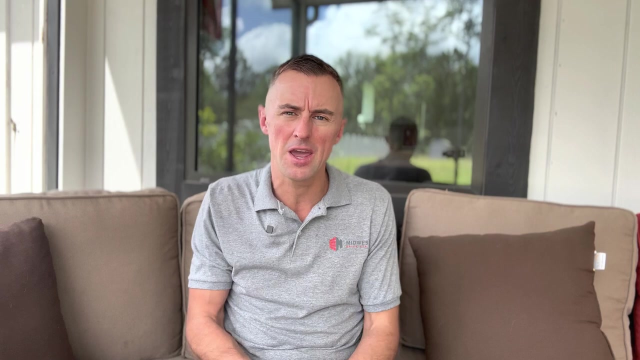 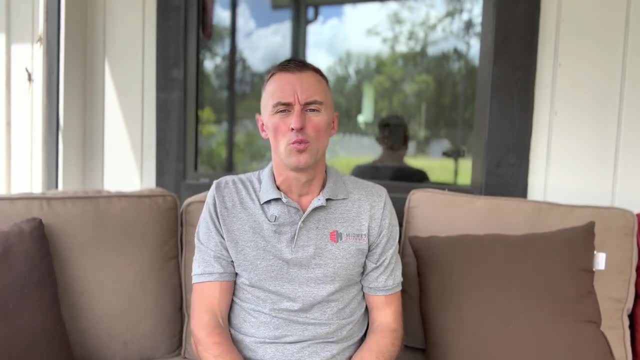 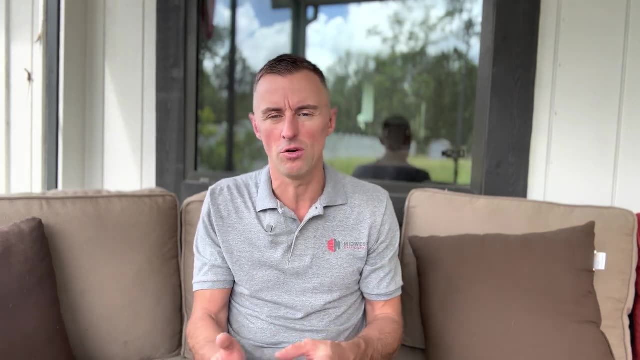 Next one I wanted to cover is we're getting more and more requests on lime-based products. Do you do a lime wash? Do you use lime products? No and no. So here's another mismarketing that some companies are using. I'm not going to mention their names. 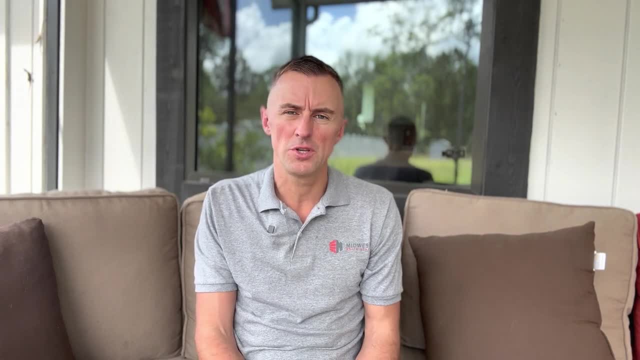 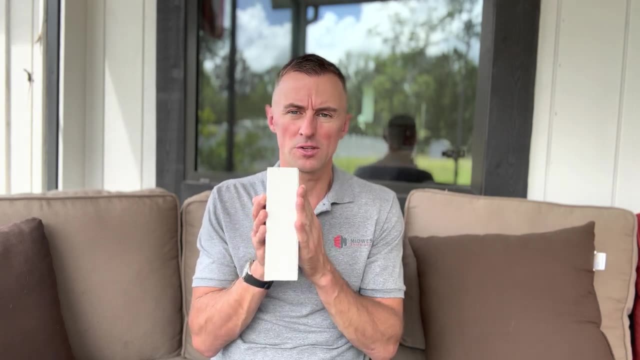 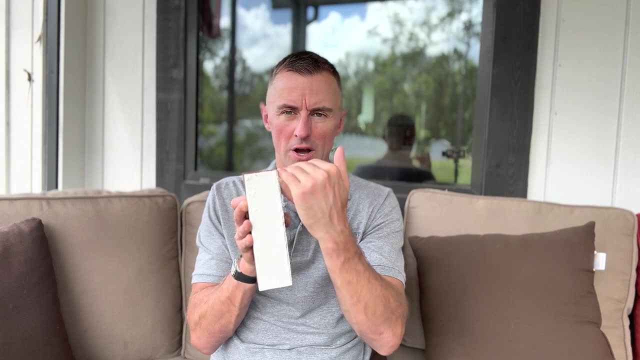 But a lime-based paint is going to achieve between a 14 to 15. ph- it's as high as it could go. so, for instance, this one is 11 to 12, another two or three ph higher. it's even that much more alkaline. what will happen with a lime based if we add these pigments? 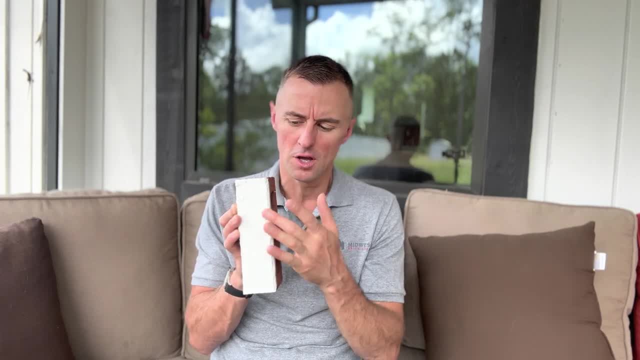 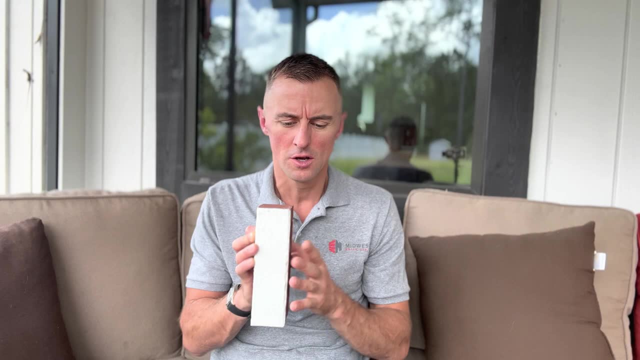 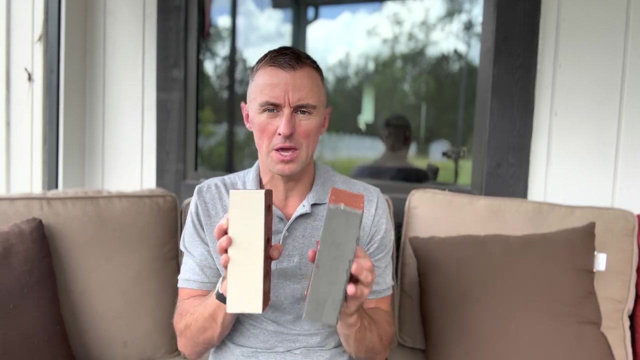 to a to a real lime based product. these colors are going to fade over time, so a lime based paint is only and it only comes in white. so when people tell you it's a lime based product and it comes in beige or it comes in maybe a gray or a darker gray like a sway, that's a mismarket and they're. 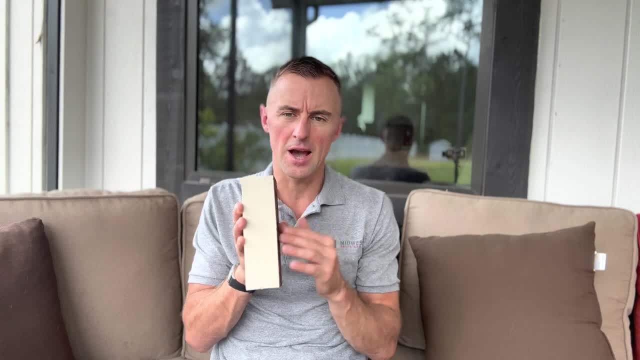 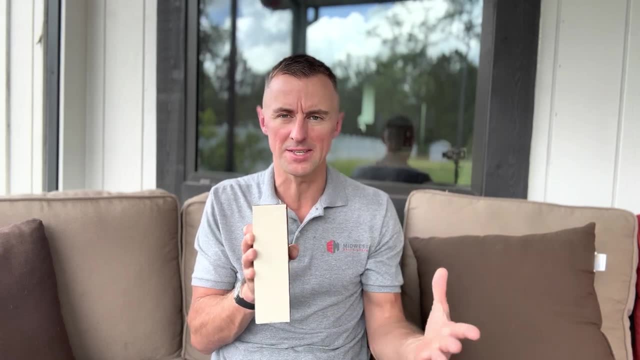 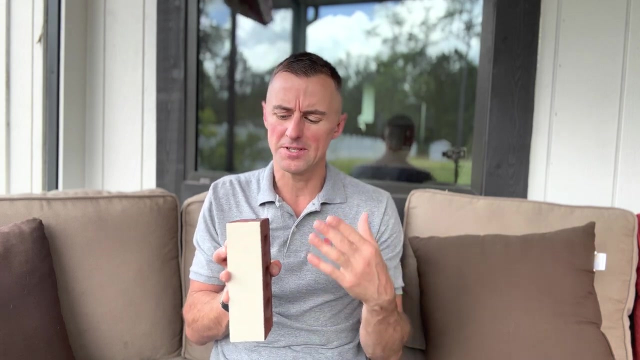 misleading you, because the higher the ph, the composition, it's going to start to break down that color, for example, and then it's going to come back to white, if that makes sense. the other thing is, if you use a traditional lime paint, if you want to call it, what happens is when you apply it, you have to impregnate it. 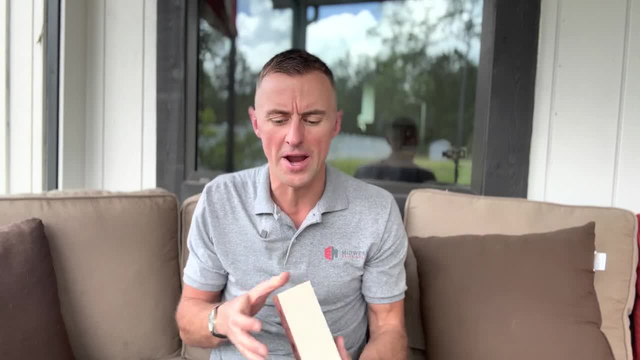 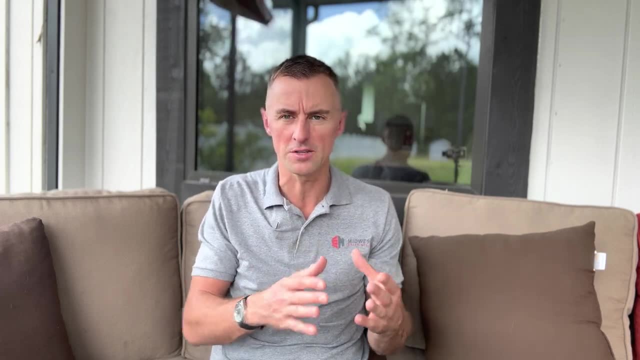 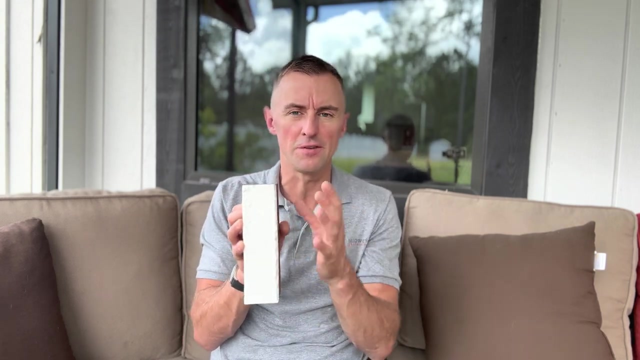 so imagine like when you put down a granite countertop, you put a sealer over it. for instance, when you actually apply a real lime product to the exterior brick, you have to put something over to protect the uv, otherwise it's going to fade within three to four seasons, maybe five max. 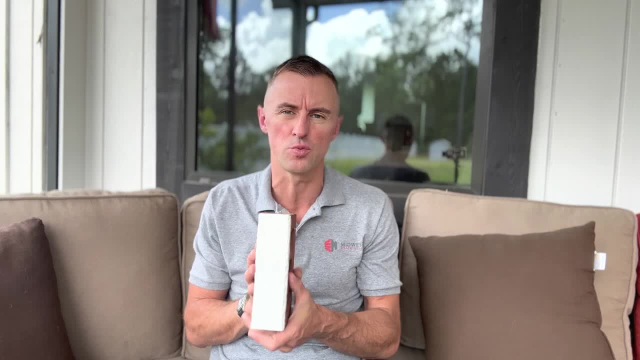 so that's another mismarketing that we're seeing out there. so i just want it to be fully transparent and cover the differences in these products.